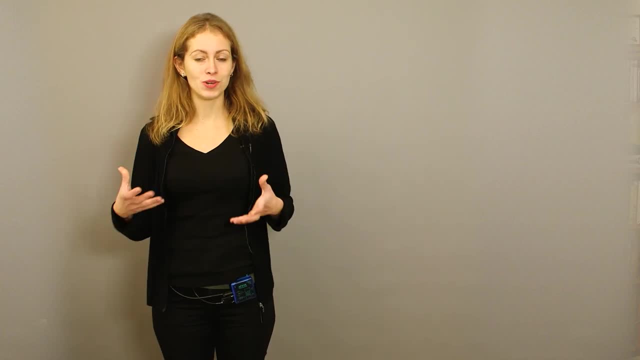 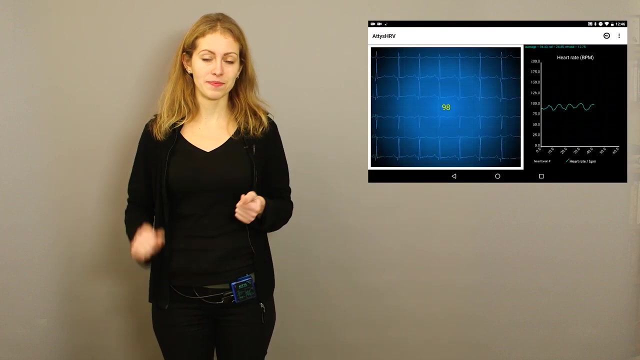 feeling the pulse on your wrist. or if you want to do it in a more precise way, then you can measure the time between two heartbeats. So, in order to do this, we'd measure our ECG first and then the time between two heart peaks. Now, why do we need this precise info? Well, because our heart rate changes. 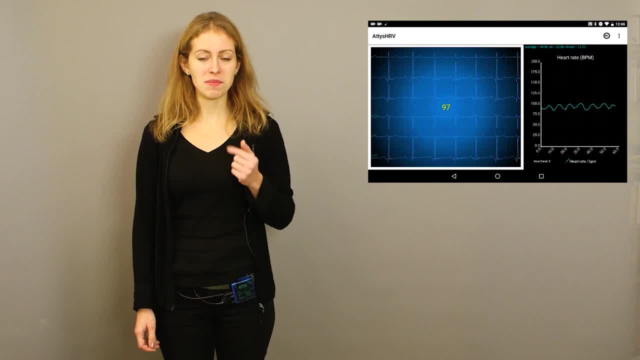 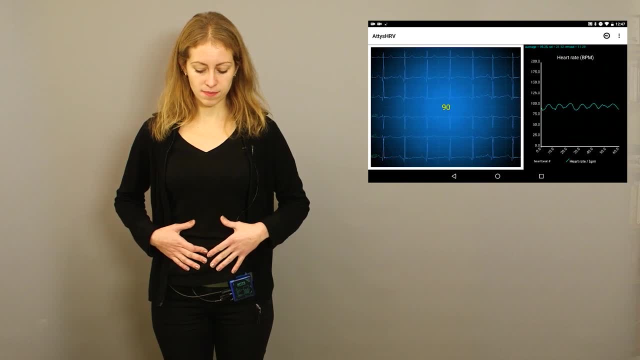 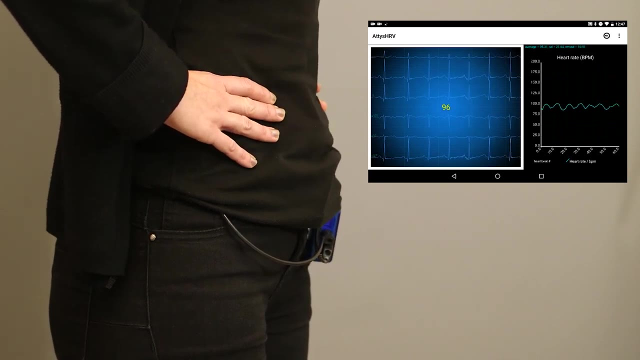 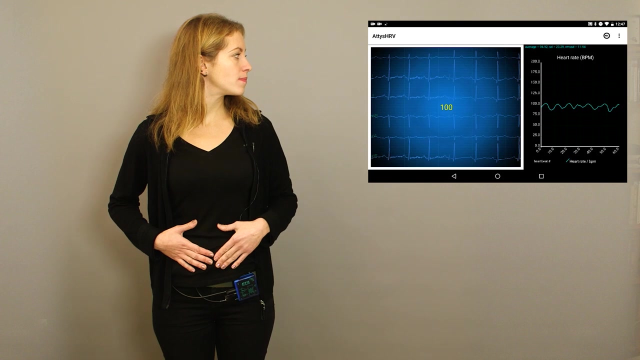 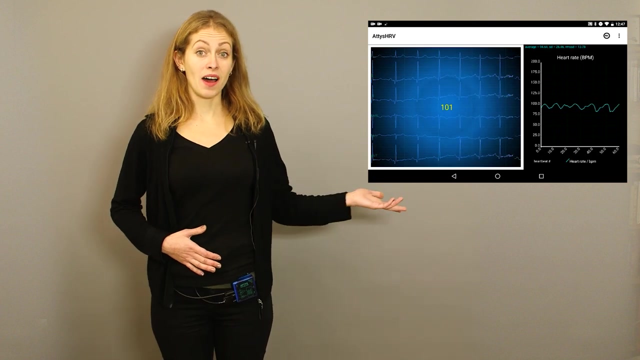 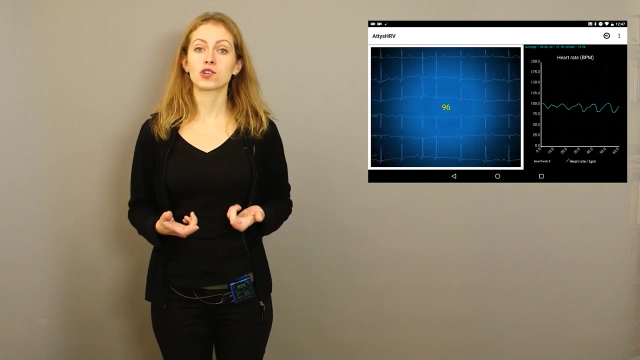 every time we breathe in and out. Let me show you an example. So, as you can see, every time we breathe in, our heart rate increases, and every time we breathe out, it decreases. This is controlled by the body's autonomic nervous system and, in particular, by 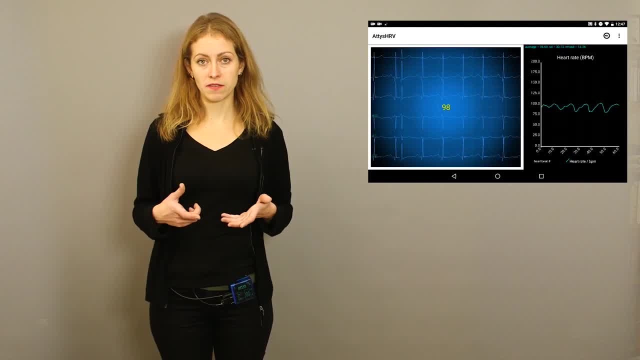 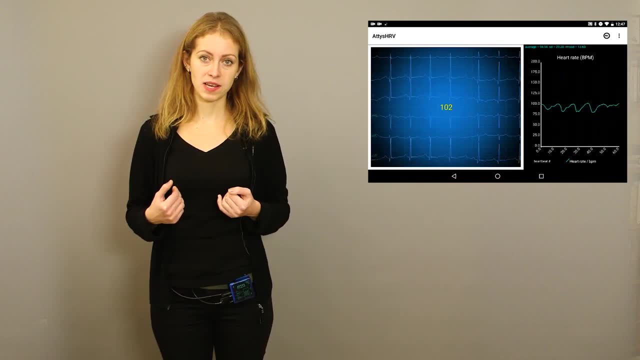 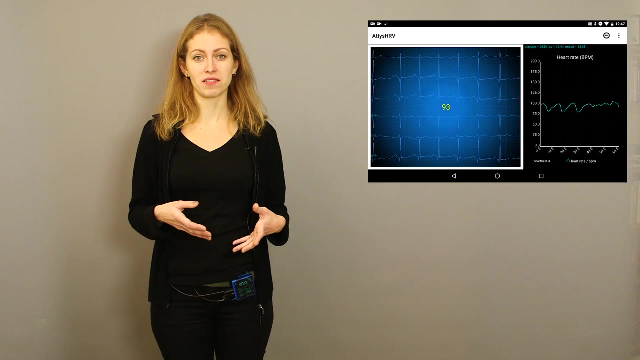 the heart rate. This is controlled by the heart rate and the heart rate level, the vagus nerve, which has a strong impact on our heart rate. In turn, the autonomic nervous system is closely linked to our emotional system, having a direct effect on our stress and anxiety levels. It has been shown that stress 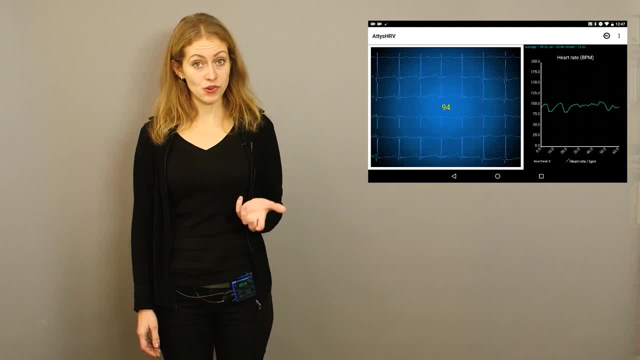 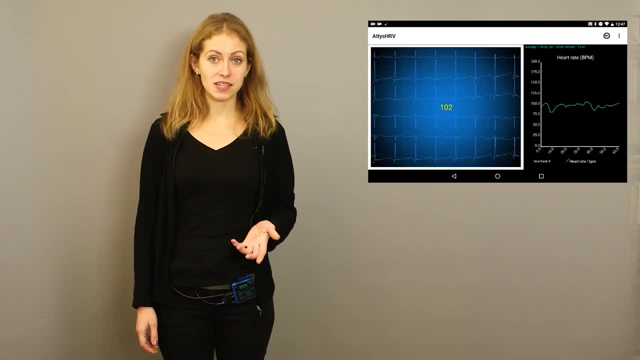 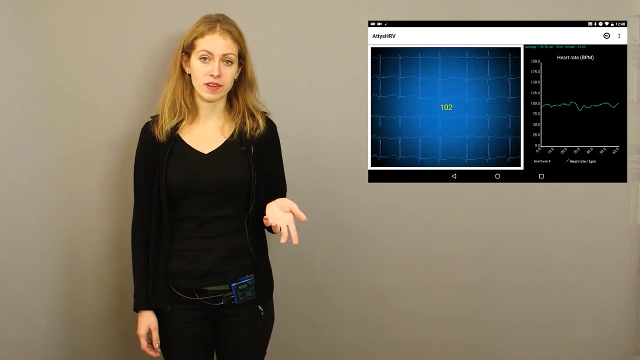 reduces heart rate variability, so stressed people will not show the sine wave like pattern. However, as I have already stated, you can use breathing, and more specifically deep breathing, to de-stress, and a good indicator for this is the heart rate variability which is plotted here. So I'm 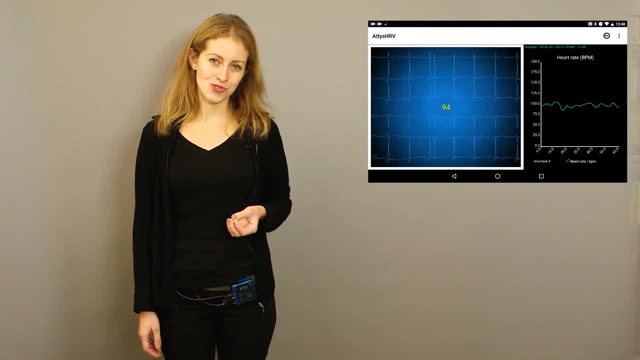 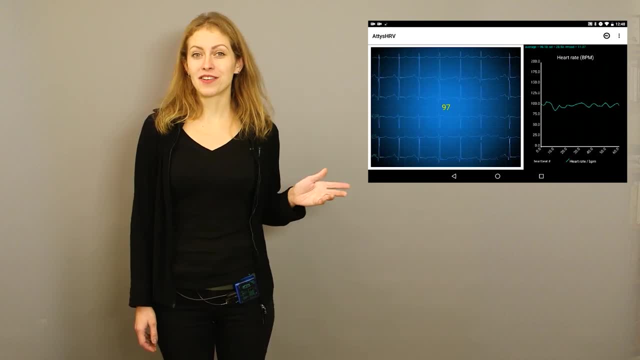 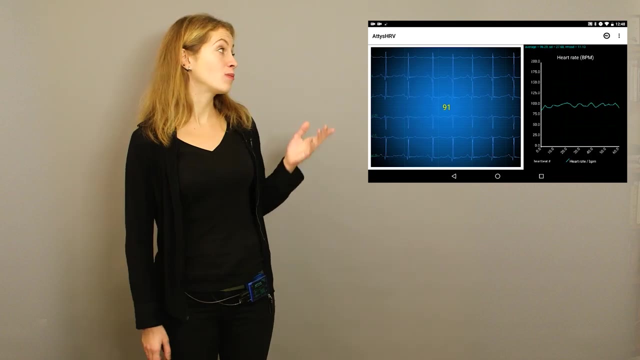 going to show you an exercise now which will help you reduce your stress levels. If you have an HRV monitor like the ATIS, then you can directly see if your HRV increases. This is a form of biofeedback. In order to make it look more relaxing, we have 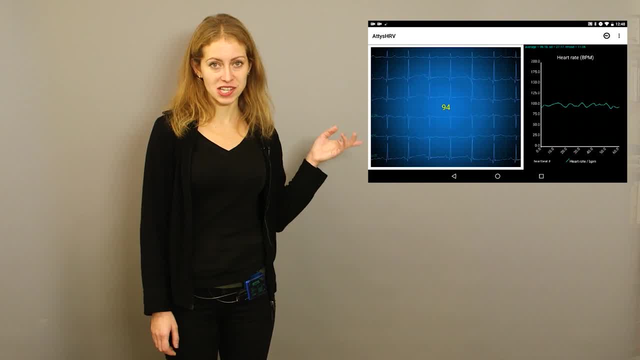 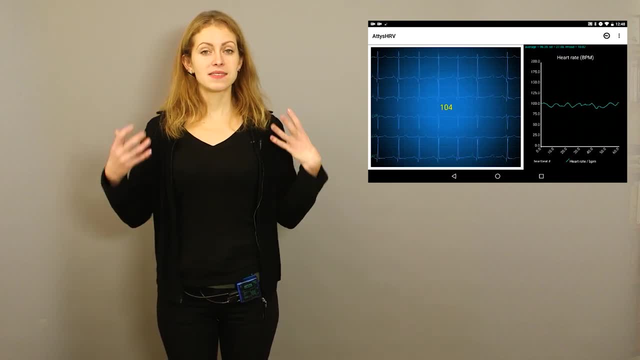 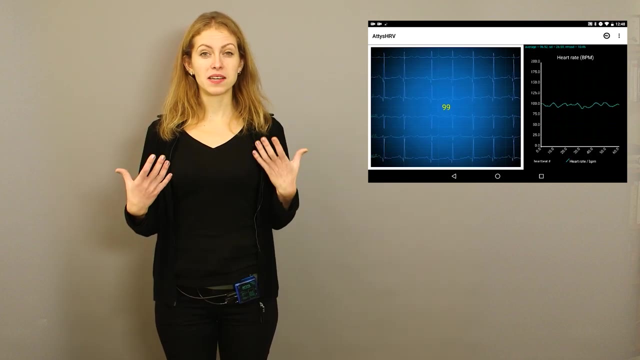 plotted the heart rate changes here as these concentric circles. So let's begin with our exercise. Please sit up straight with your spine erect but not stiff. Let your shoulders drop and try to release any tension from your arm and back muscles that you might be aware of. Keep your head above your spine.